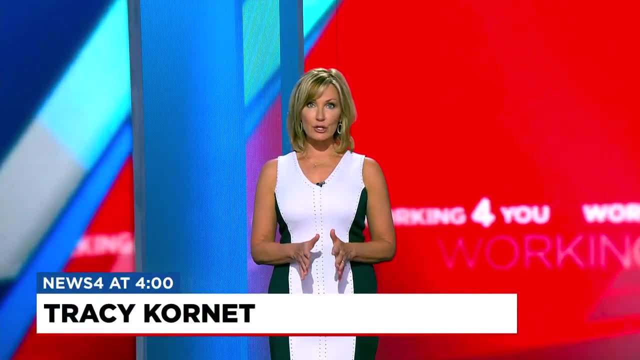 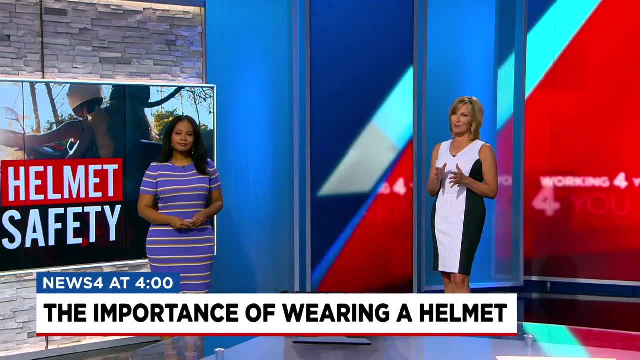 Kids and teens enjoy their summer. Doctors are encouraging and urging parents to make sure they're wearing the proper safety gear. We're in particular talking about helmets here. Newsforce Alexandra Adams joins us now live Alexandra. we know the Children's Hospital at Vanderbilt already seeing a. 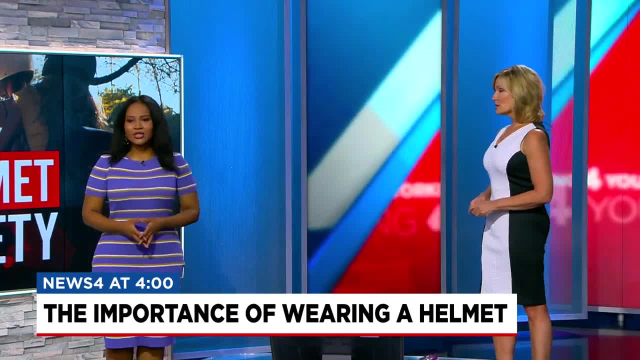 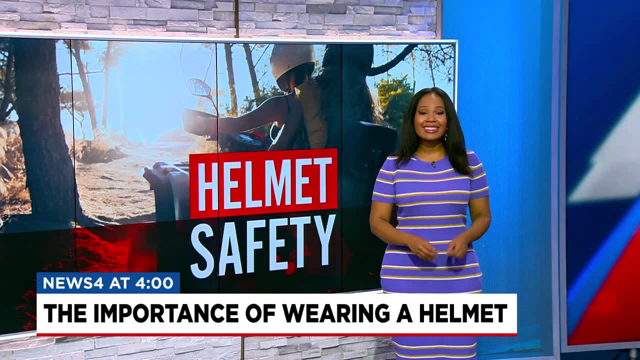 lot of head injuries. They are devastating, They really are, Tracy, Yeah, they want to put a stop to that, And the best way to do that, of course, is to wear helmet. We spoke with the mother and her teen daughter, who had to. 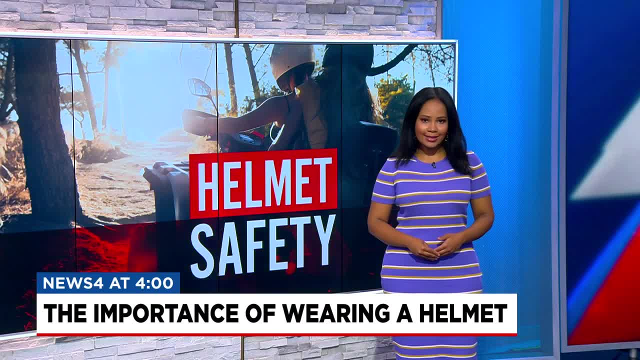 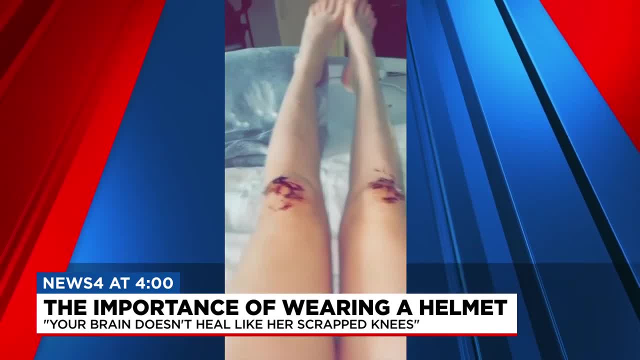 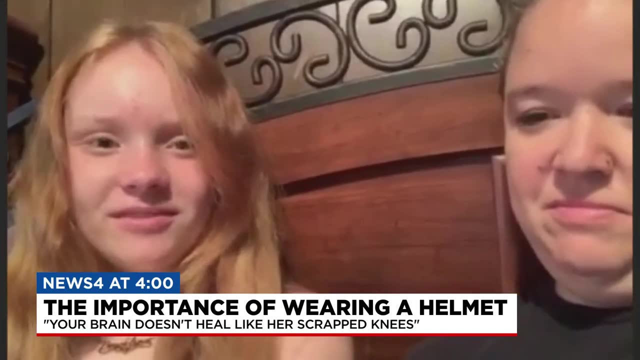 be lifelighted to the hospital after a scary A T V Accident. This is 14 year old Brooklyn Sutton. just a few weeks ago out playing softball And this was her last week inside of the Children's Hospital at Vanderbilt After an A T V Accident. I was trying to turn to the children even. 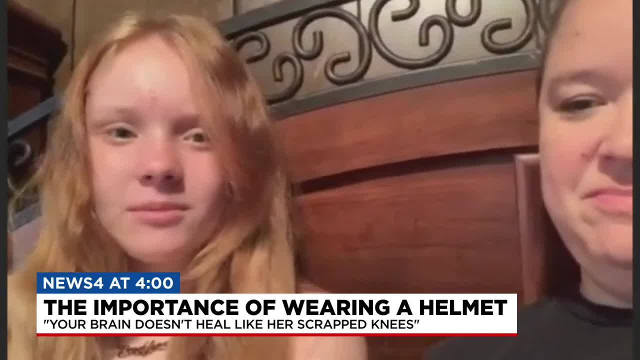 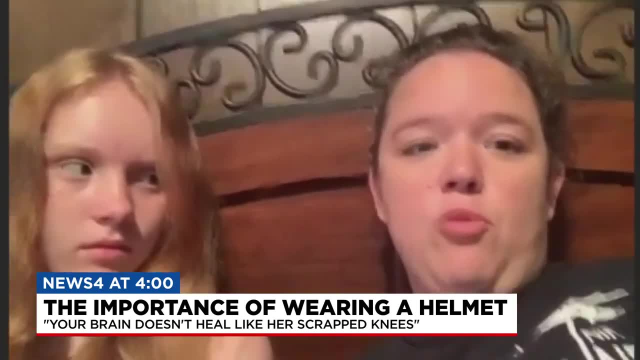 though I passed it and I was going 40 and it flipped 12 times. Brooklyn was flown by lifelight from her home in West Tennessee, two hours away from Nashville. It was a lot more than just a little cut on her head. Um, instantly, just just fear. 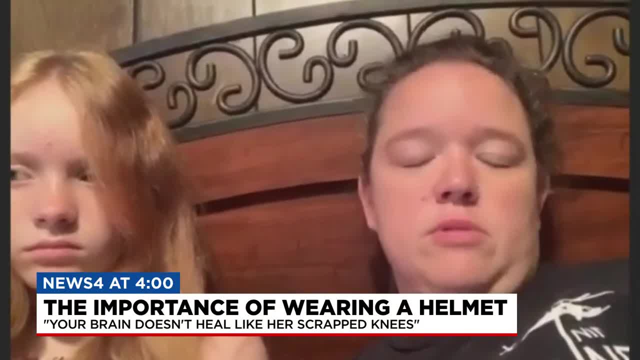 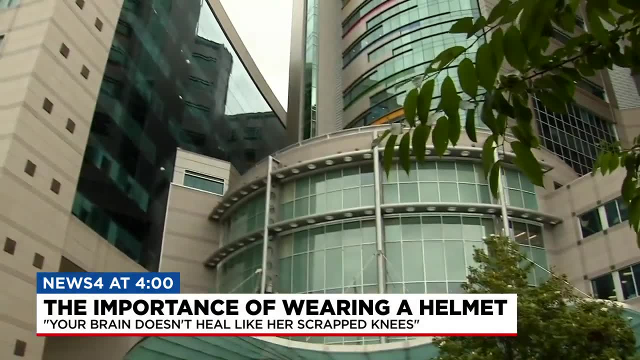 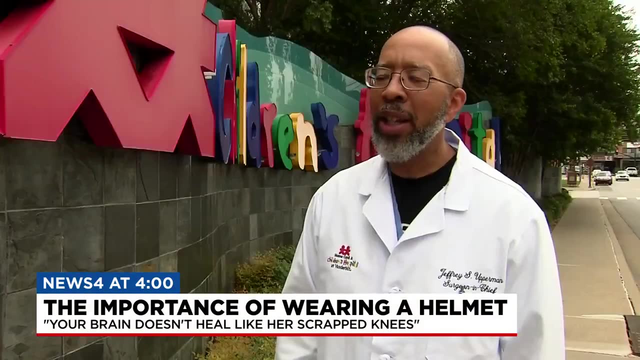 and panic, Not knowing is absolutely terrifying. as a mother, Brooklyn had bad injuries, bruises, road rash and a concussion. Doctors at Monroe Carol Junior Children's Hospital say they're worried they're going to see more cases like this. We see a T? V Crashes all the time. We see actually very 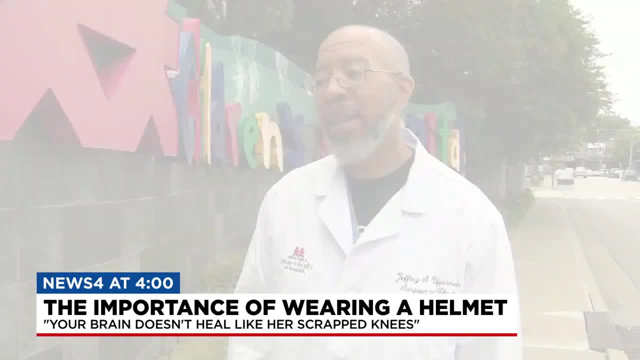 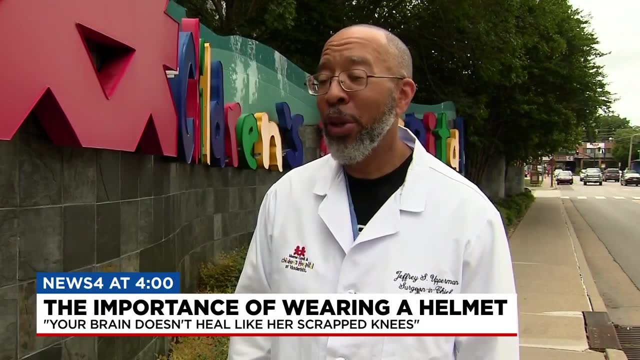 seriously twice a week And so we're seeing those numbers go up. As a father, I would tell them: don't get on an all terrain vehicle. But I understand that we're in Nashville, Tennessee, and we're a rural state and folks are going to have them around the farms and other areas While she may. 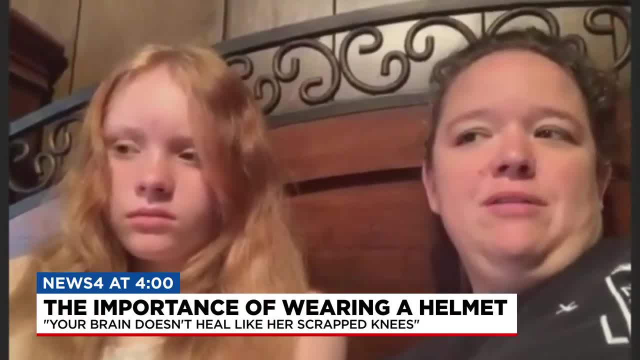 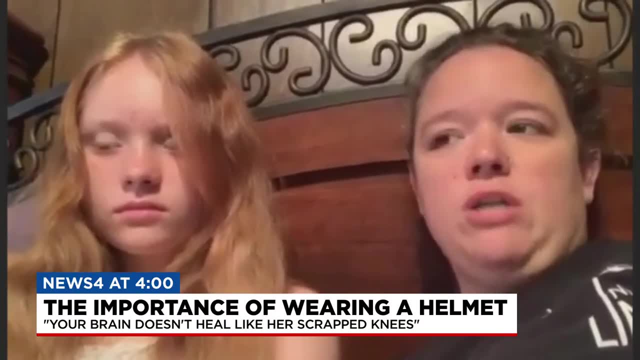 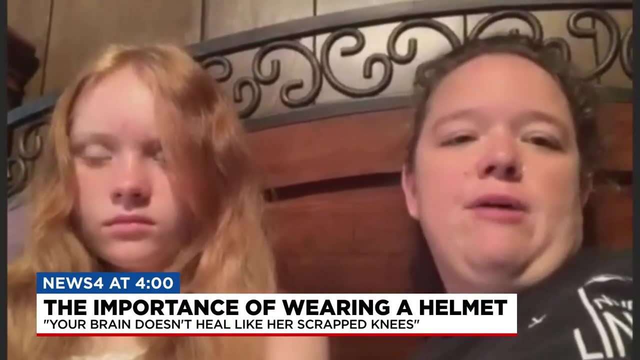 look well on the outside. Brooklyn is still recovering. Your brain doesn't heal like this. You know her knees scrapped, scraped up knees, and it's been hard on her. you know watching her sisters and everybody else go to softball practice, go swimming. you know running and playing outside. 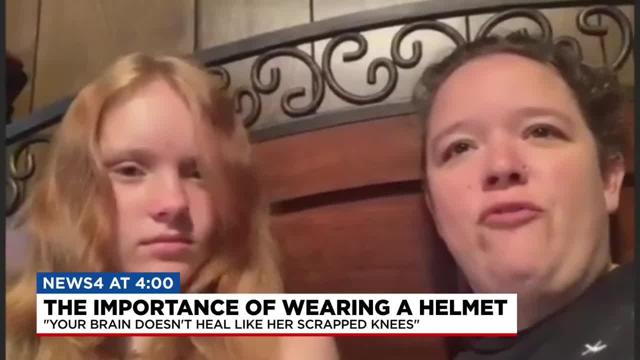 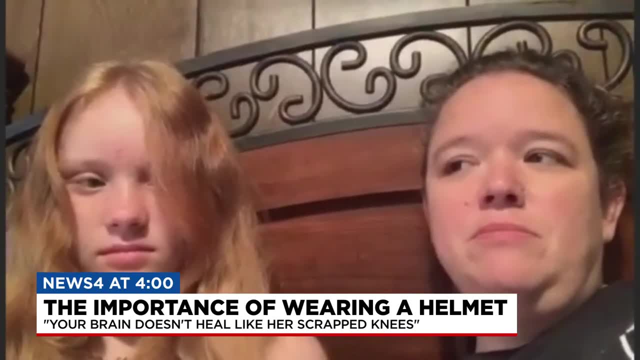 Brooklyn says she has no plans to get back on an A T V. Her mom wants other parents to encourage their kids to always wear a helmet. as a mom, You know, and I tell the kids: no, it may not be cool, but your life is worth more.